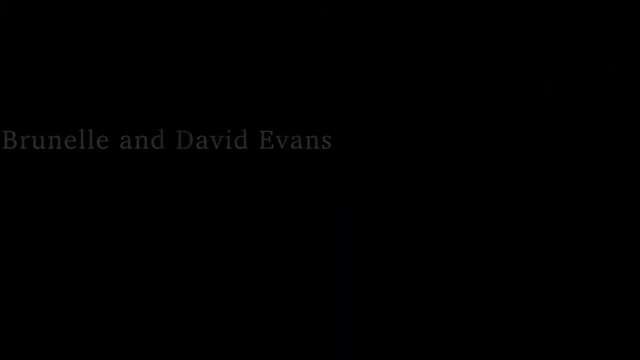 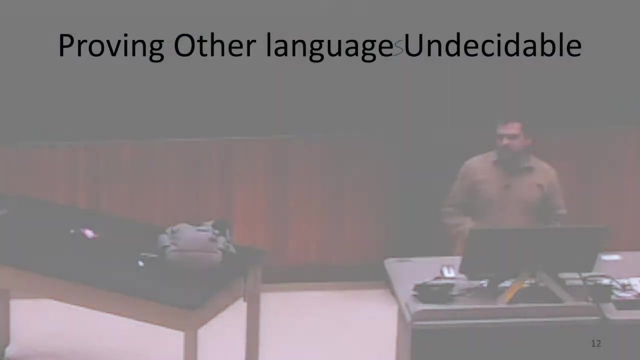 What we're going to do next is we're going to find some way of proving that other languages are undecidable. So we have two of them. We have two non-computable languages or non-computable functions: halt and accept. Both of those were proved in kind of the similar way. We had a very 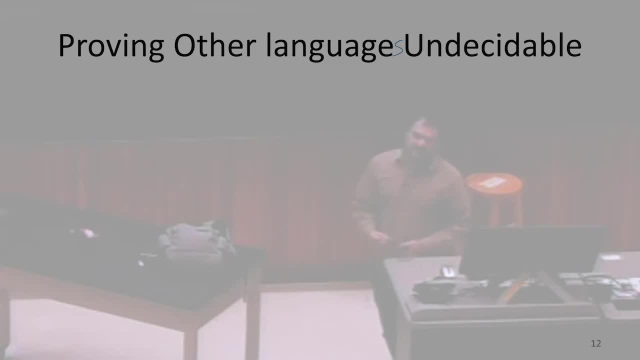 similar contradiction for both of those last class. What we're going to talk about today is how we can do more. Those contradictions are not something that is going to be easy to do for extra languages. Those are sort of special languages or special functions that lend. 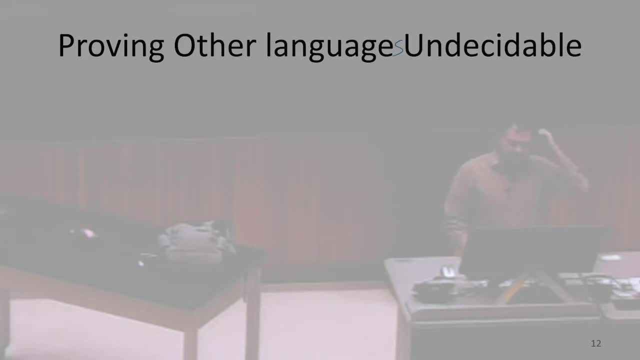 themselves to that sort of contradiction. What we're going to be talking about today is a more general way of proving more languages to be undecidable, And the technique we're going to use for this is something called a reduction. The idea of a reduction is that we can show relationships between two entirely different 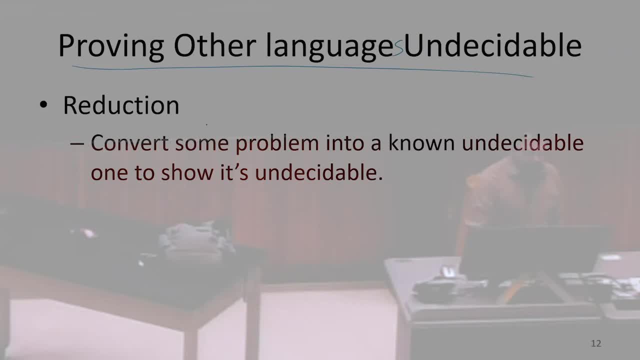 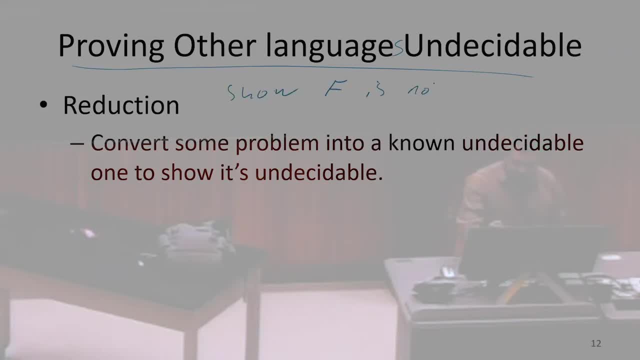 So to show f is not computable, we're going to, in a special way, relate f to, let's say, f prime, which isn't computable, which we somehow already knew wasn't computable. So we're going to be leveraging our knowledge that some function, f prime- wasn't a computable. 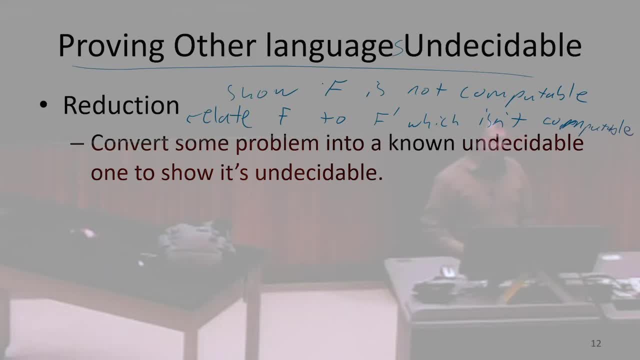 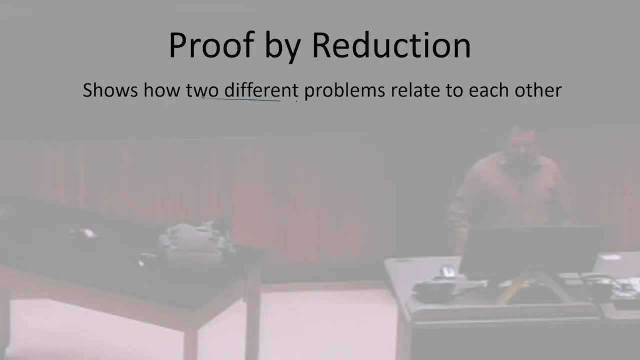 function in order to show that this new function, f, is not computable. So the idea of reduction is just show how two different functions relate to one another. So in order to demonstrate this, we're going to watch a little bit of a movie. 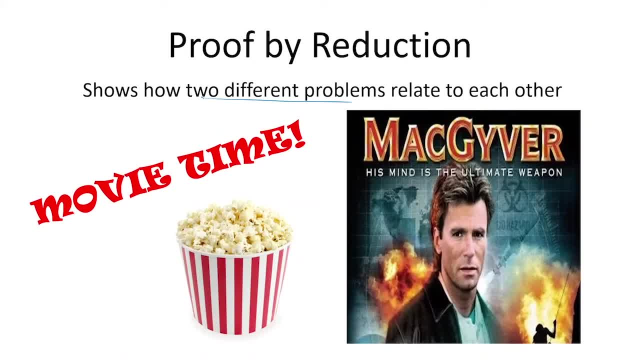 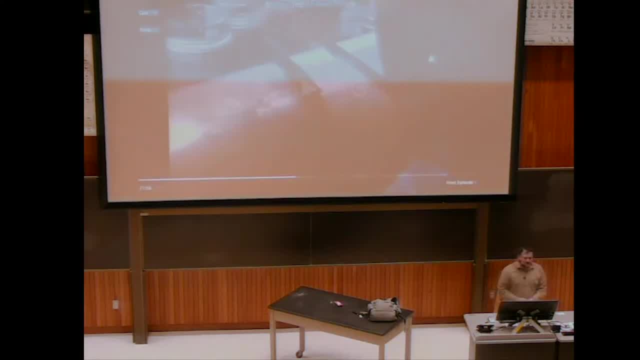 I got jealous. I got jealous of Professor Evans showing you a movie last class, so I decided that I'm going to show you a movie this class too. This is from a TV show from the 80s called MacGyver. 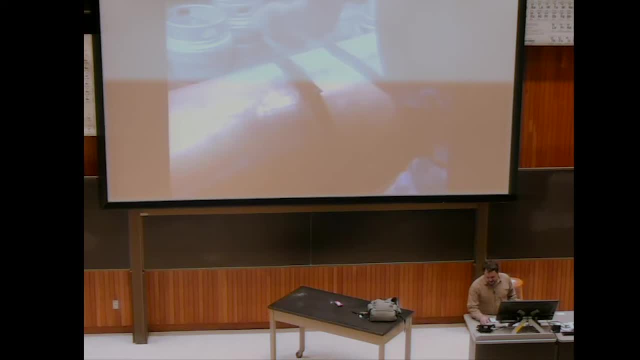 Basically, the premise of this TV show is that there is this guy who catches bad guys and finds himself in these impossible situations where he uses his own ingenuity and just the resources around him to get himself out of those situations. So the setup for this scene is: MacGyver has been knocked unconscious. 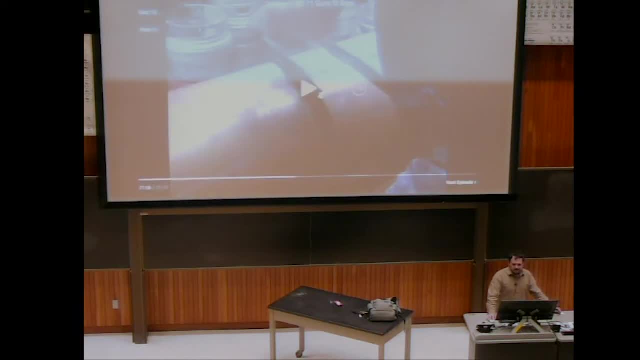 And then thrown into the storage closet of a bar by the bad guys, and they locked him in there. He's got to figure out how to get out. So what he's done is he's found a piece of duct that was just laying around conveniently. 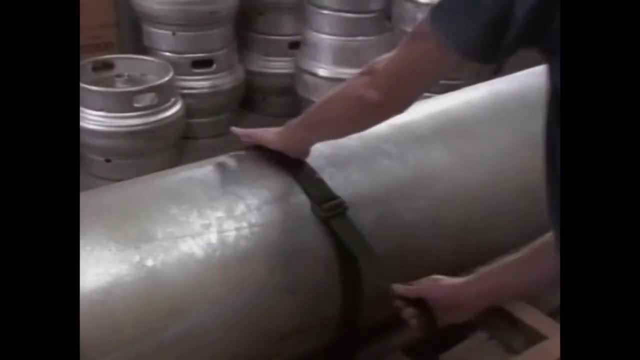 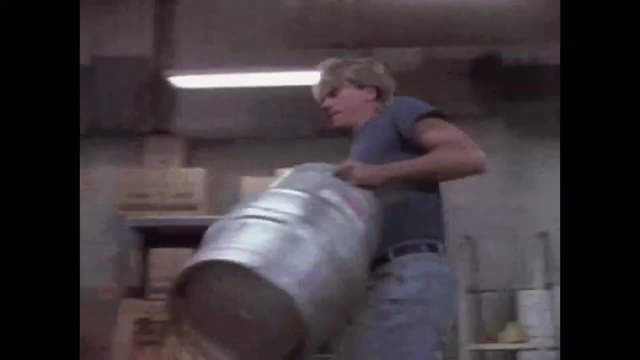 and he's strapping that to the floor. And now, since he's in the back of a bar, this is a keg of beer that he is putting into that duct, And it happens to be a perfect fit. And now, since he's in the back of a bar, this is a keg of beer that he is putting into that duct, and it happens to be a perfect fit. 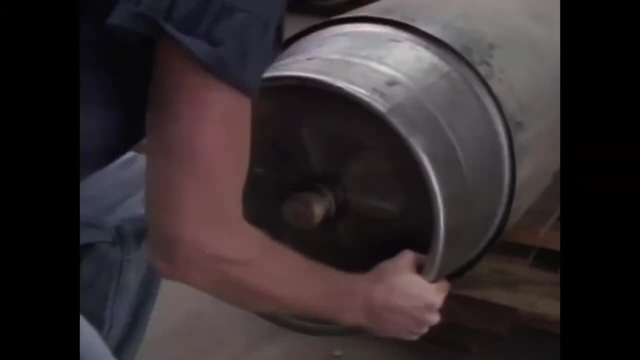 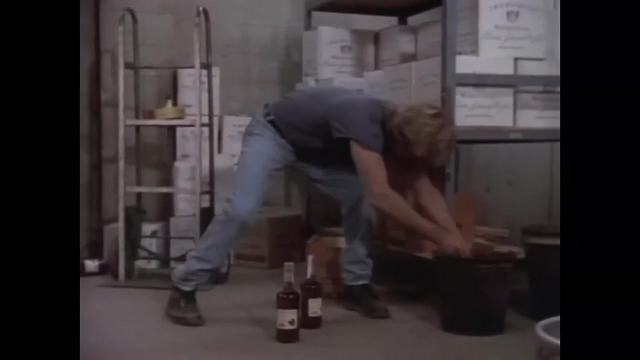 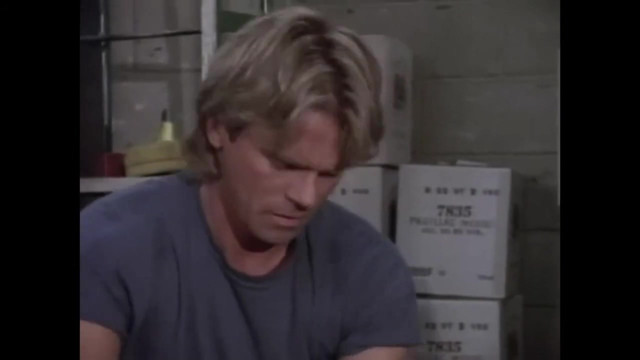 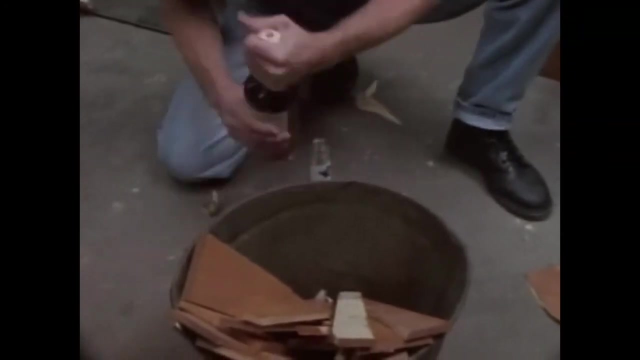 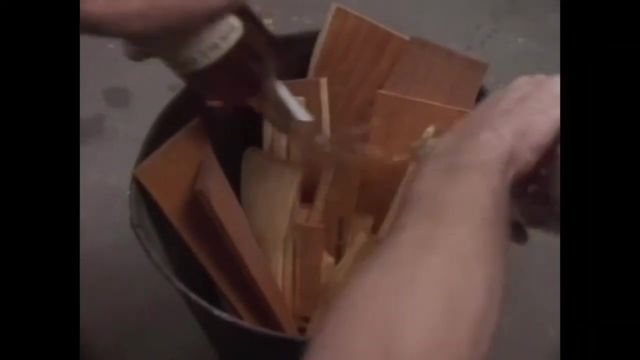 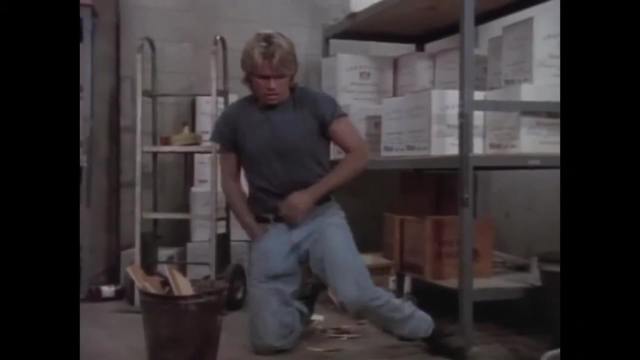 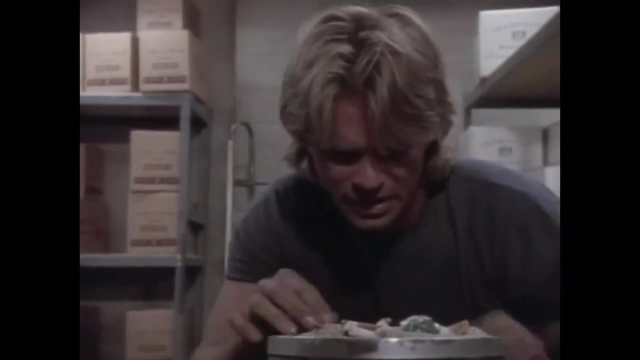 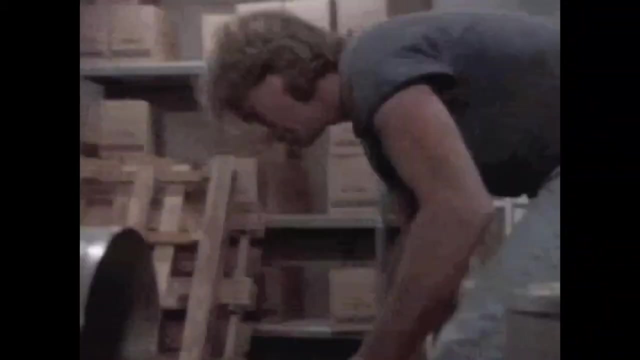 And now, since he's in the back of a bar, this is a keg of beer that he is putting into that duct, and it happens to be a perfect fit. That is some high proof alcohol He's dumping on the wood, Followed by the world's most convenient book of matches: the 80s music intensifying. 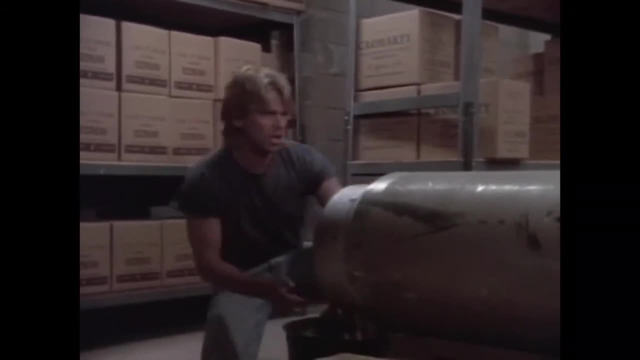 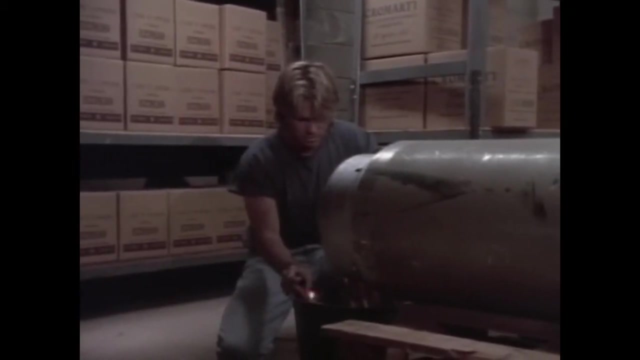 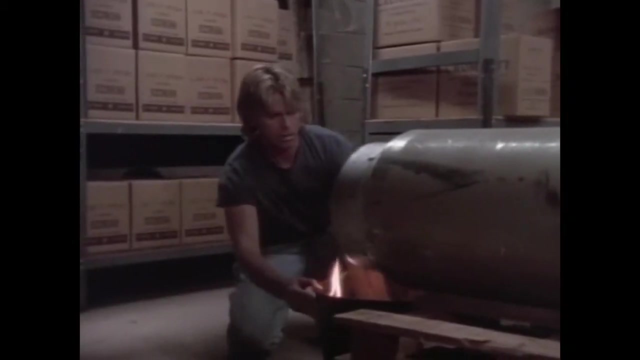 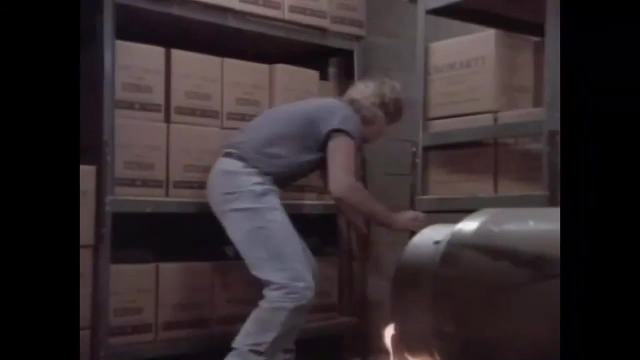 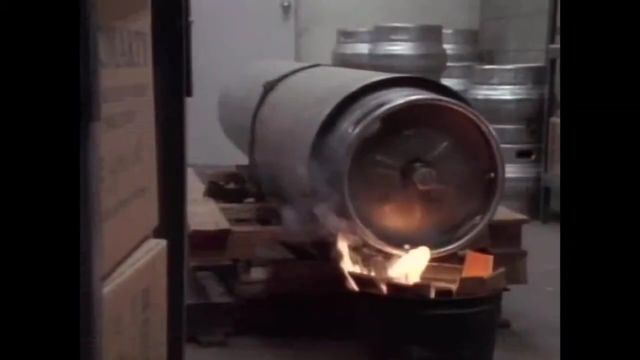 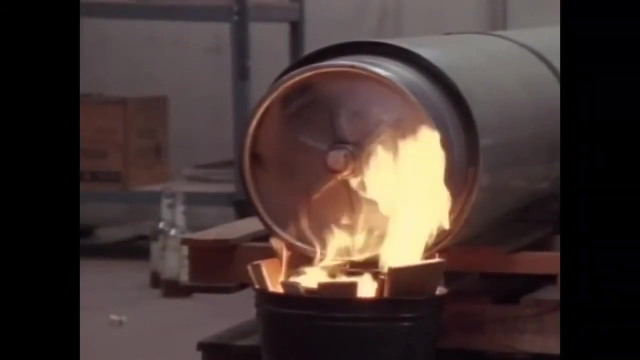 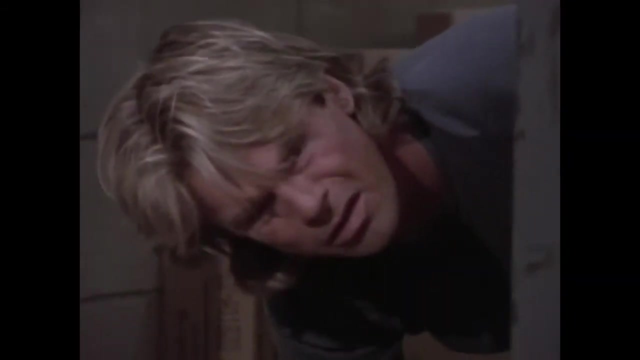 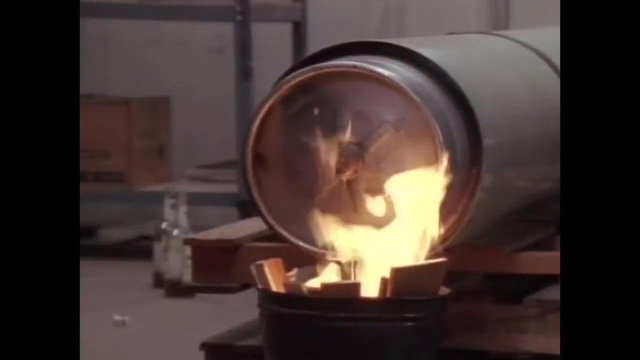 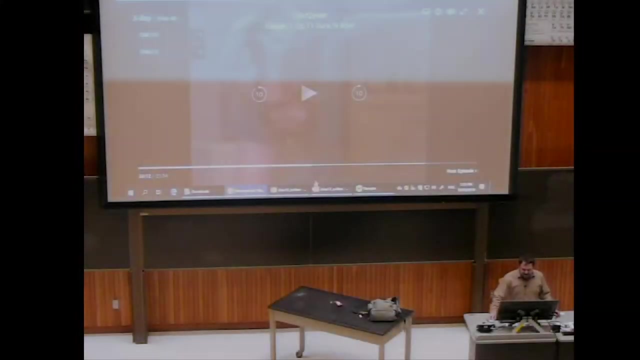 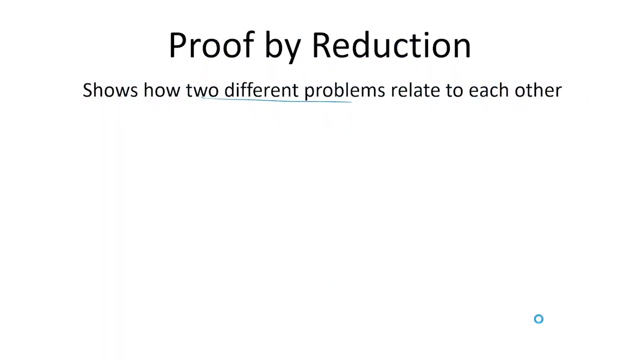 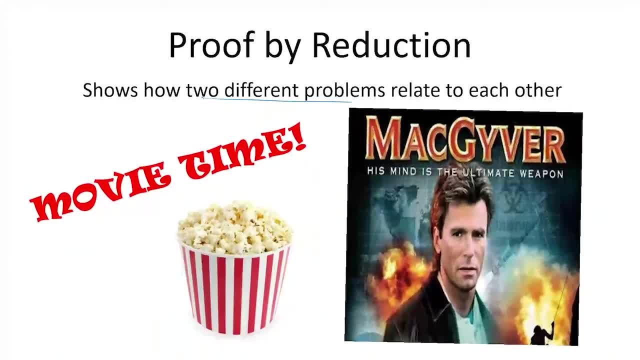 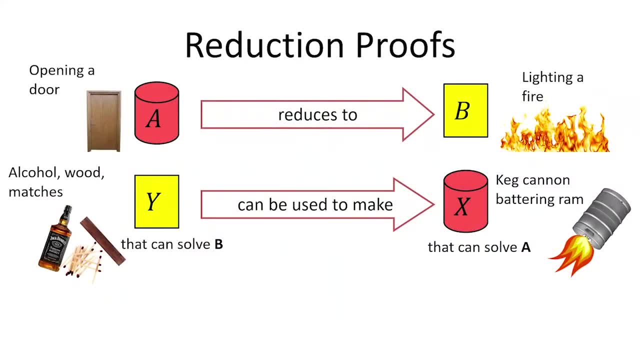 So MacGyver had to open a door. He had this problem. he was trying to solve this function. he needed to compute which was this opening a door function. And what he did is he converted that, He related that or reduced it to this different problem, this entirely different problem, that of lighting a fire. 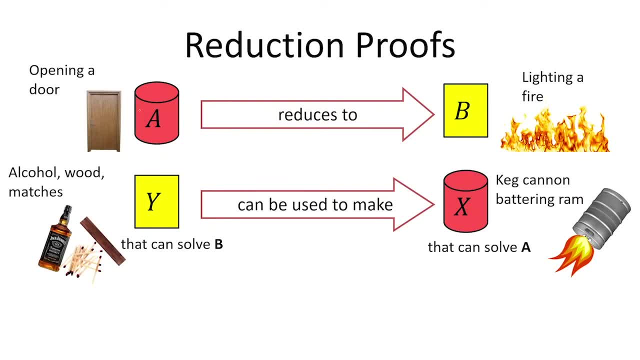 So he reduced the problem of opening a door to that of lighting a fire, And the way he did that was he provided a function that would kind of do that conversion for him. So he showed that the problem of opening a door can be converted into the problem of lighting a fire. 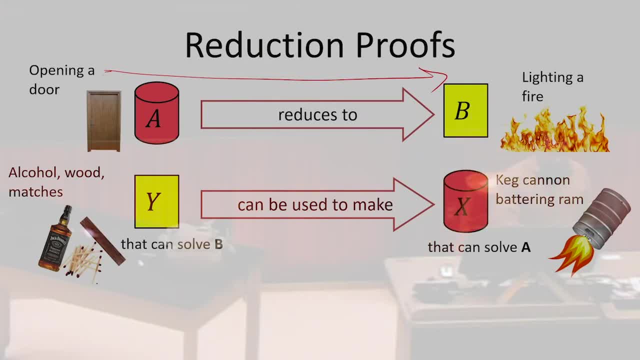 And the way that he did that is by showing that some way that I could light a fire. in particular, the way that he used was alcohol-wooden matches, So he had some way of lighting a fire. He showed that that could be. 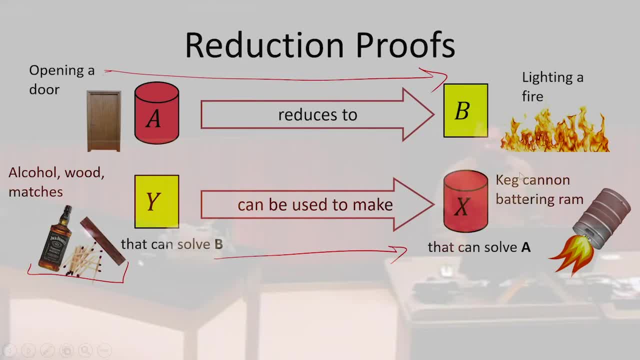 That could be used in order to build this Keg Cannon battering ram, which ended up being a solution to opening a door. So Keg Cannon battering rams that opens doors. So the problem he needed to solve was opening a door. 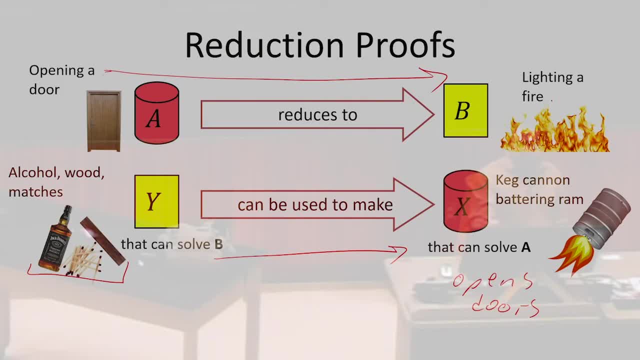 The way he decided to solve that was by reducing it to lighting a fire, because he knew that by solving this lighting a fire problem he could produce a Keg Cannon battering ram and have a- now handy door opener. So the way that we're going to use this idea of reductions is to in some sense compare the difficulty of two problems. 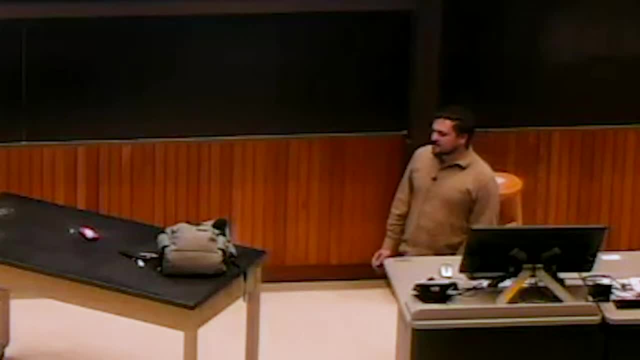 Undecidable problems, non-computable problems. we're going to consider those to be really, really hard to solve. Non-computable functions are hard functions to compute, So we're going to show other functions are non-computable by using reductions in order to show the relative difficulty of these problems. 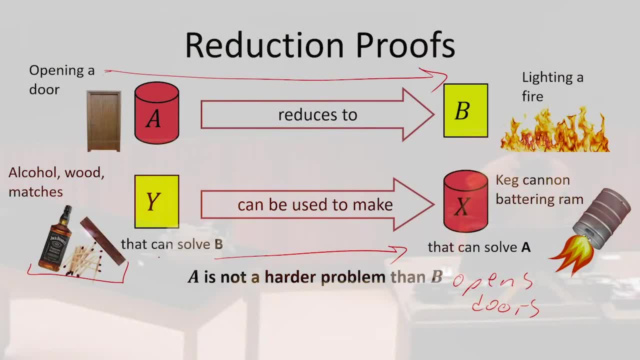 So what we showed, What we show here, is we show this problem A of opening a door is not a harder problem to solve than that of lighting a fire. So basically the idea here is: as long as I had some way of lighting a fire, I don't care which way it was to light a fire. Alcohol, wood and matches seems to work. If I happen to have gasoline that would probably work too. But any way I have of lighting a fire that can be used to build a Keg Cannon battering ram. MacGyver showed us that. 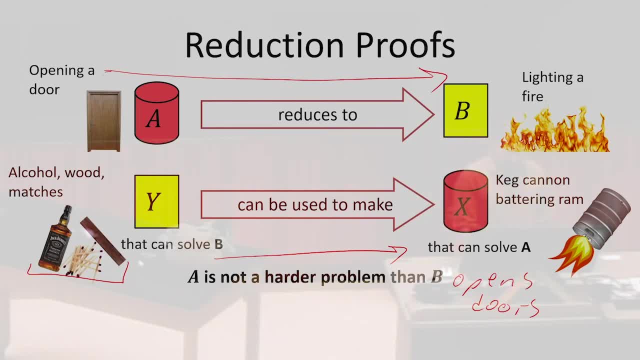 He proved that to us. So that means that, assuming I can light a fire, opening a door is easy. So, assuming I can light a fire, opening a door is easy. This also means that if I somehow already knew, if I somehow totally believed that opening a door was really really, really hard to do, 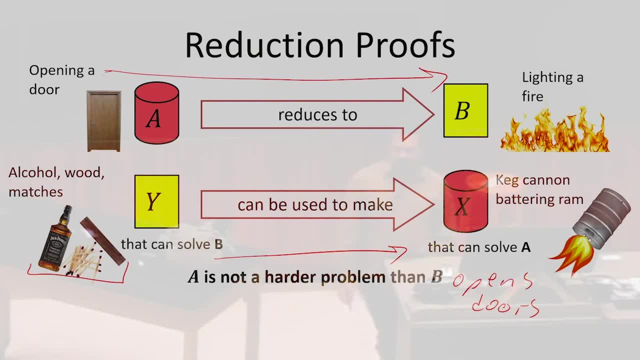 I must also be able to conclude that lighting a fire was going to be hard to do, Because if I could light a fire easily, I could open a door easily. So if opening a door was hard, lighting a fire must also be hard. 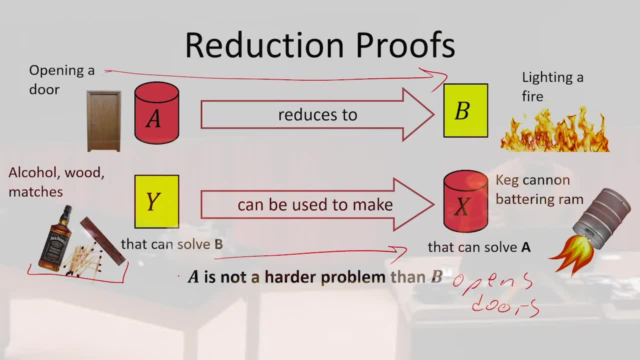 So this is how we're going to use this idea of reductions. So, because we could solve opening a door by solving lighting a fire, I knew that this problem of opening a door was not substantially harder, was not really any harder than that of lighting a fire. 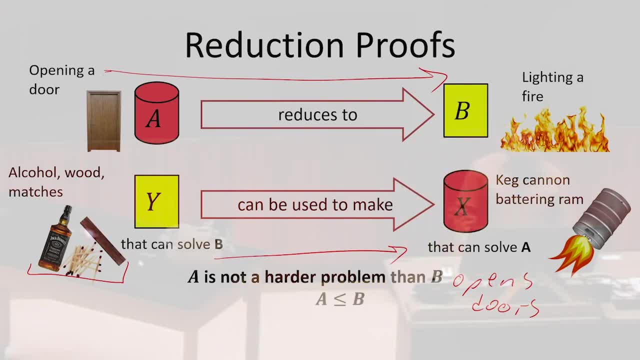 Lighting a fire was sufficient for opening a door. So what we're going to do is, if I have this problem, this function, this language, something like that, let's call this A, If I can reduce A to B. pay very careful attention here. 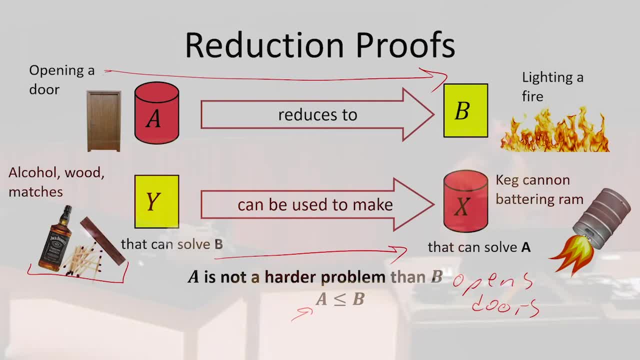 This might look backwards, but it's correct. If I can reduce A to B, then that means the difficulty of A is less than or equal to the difficulty of B. So oftentimes the way we denote these reductions is that we're going to have to do something about it. 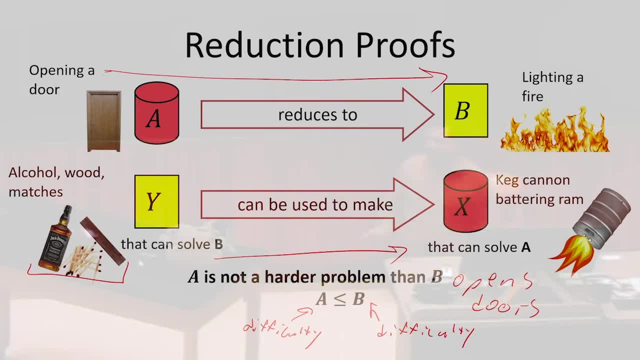 A is, with this, less than or equal to sign. that is kind of comparing the difficulty of computing those two things. So the difficulty of computing A is less than or equal to the difficulty of computing B, because A reduces to B. So what we're going to do is we're going to be proving the impossibility. 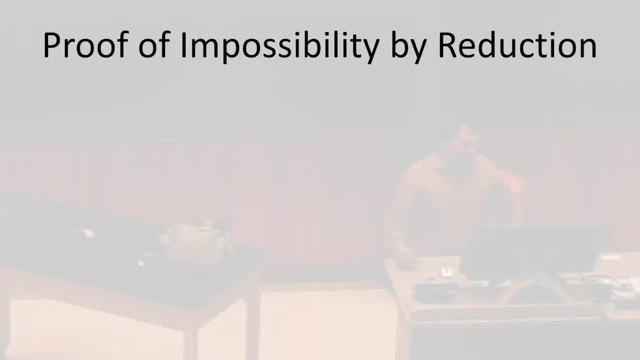 or the non-computability of certain functions using this idea of reductions. So let's say that I had a problem that I knew was going to be impossible, possibly difficult, For instance, opening a door. So opening a door is something that. 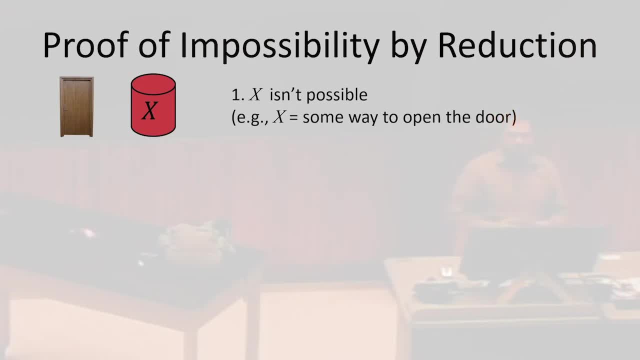 let's say that I was somehow totally convinced- the bad guy was totally convinced- that it was going to be impossible for MacGyver to open that door. So here we have something we knew to be impossible. What we're going to do is, if I have this reduction, 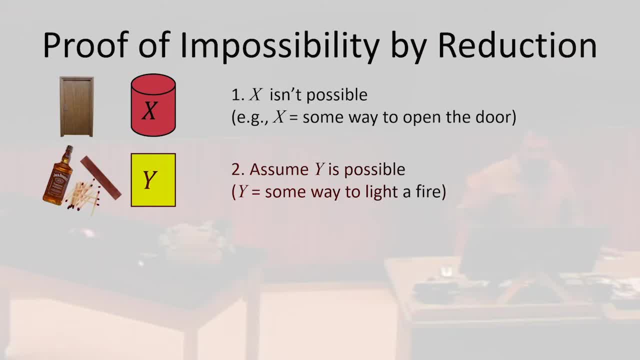 if I had some way of solving this separate problem, for instance lighting a fire. So let's say I had method Y for solving lighting the fire Because I had this reduction where I could actually take my solution Y to the lighting a fire problem. 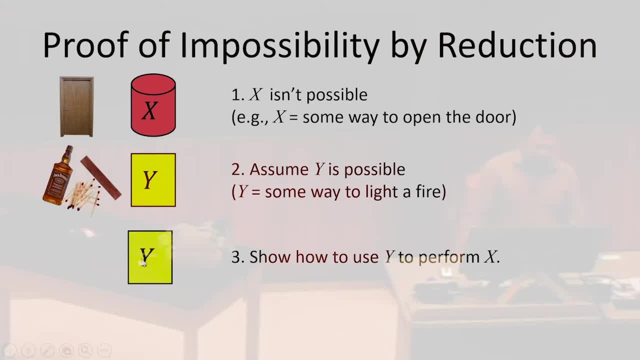 and I could do some sort of weird maneuvering in order to convert it to some solution for the opening a door problem. Yeah, I know unnecessary PowerPoint animations, But if I could show some way of manipulating this solution to Y to become a solution for opening a door. 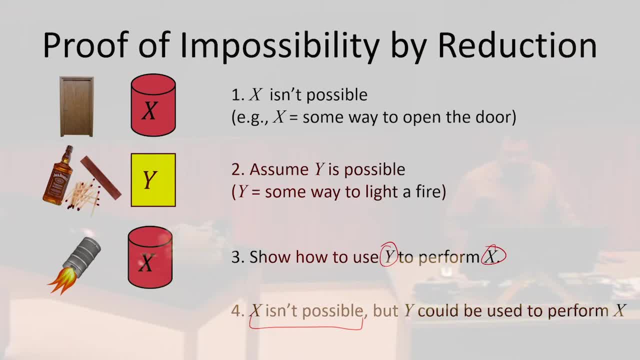 then, since I knew X wasn't possible, and once I had a solution for opening a door, and once I had a solution for opening a door and once I had a method for using Y to perform X, I must be able to conclude: Y isn't possible either. 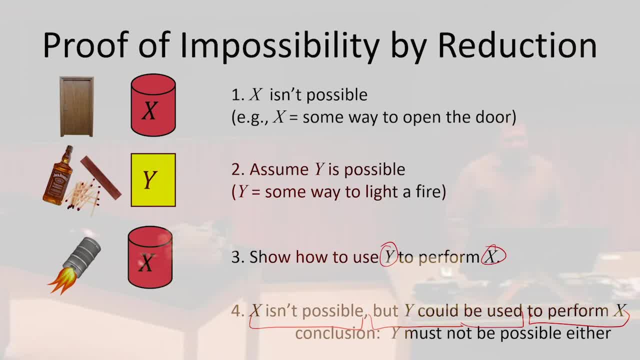 So this is kind of a fancy proof by contradiction, a special kind of proof by contradiction that we're seeing here. We knew that X wasn't possible. This is something we knew. coming into this, Let's assume, towards reaching a contradiction, that Y is possible. 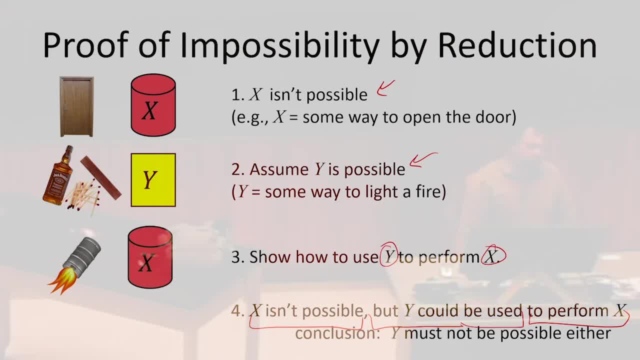 Because I had this reduction, where a reduction says I could use Y to do X. I could use Y to solve X. So if I had some way of using Y to solve this problem- X- then, since I knew that X wasn't possible. 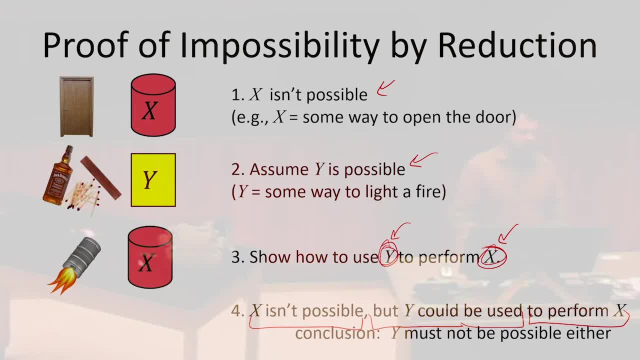 I must have been wrong in my assumption that Y was possible, Because otherwise I could have used Y to build my keg can and battering ram and solve X. So therefore our conclusion is: Y is not possible. Let's say that I'm the mob boss, or something like that. 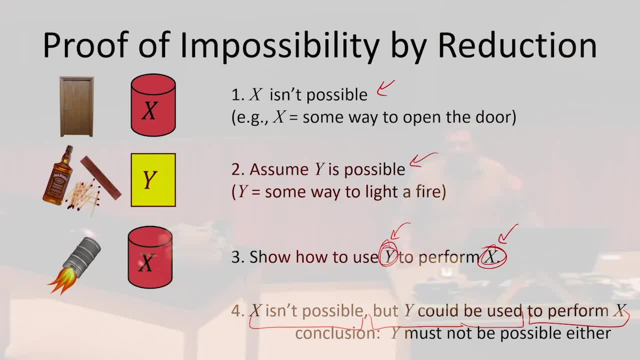 So I'm telling you, my henchman, to lock MacGyver into the storage closet, And you have convinced me as the mob boss that it is totally impossible. You've just definitively proven factually that it is totally impossible for MacGyver. 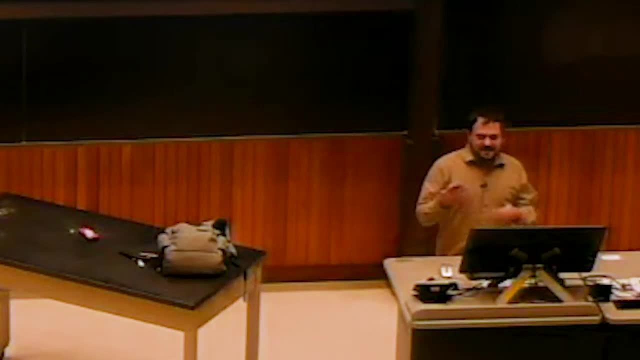 to break out of that storage closet that has things like kegs and so forth. Then somewhere along the line, I must have also been convinced he couldn't light a fire. So if we were like, let's try this again, I want you to again lock MacGyver into that storage closet. 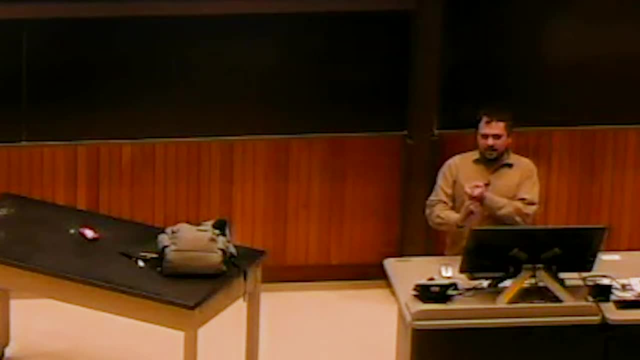 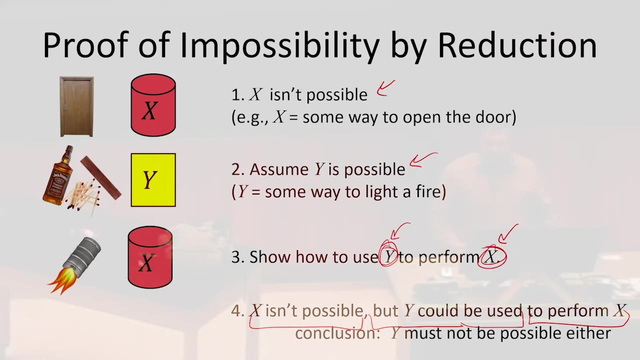 If you locked him in there with matches and high-proof alcohol and wood, then he could get out of there by building a keg can and battering ram. So if it's definitely impossible for him to get out of there, then necessarily it must have also been impossible. 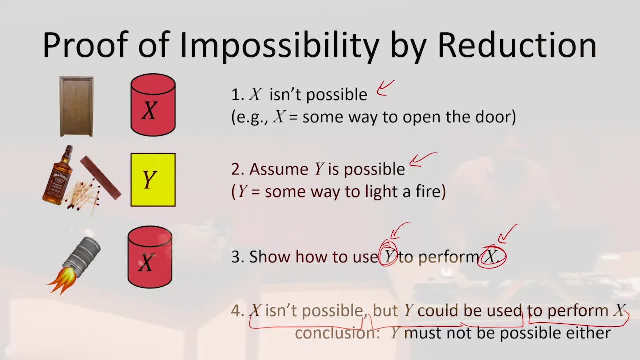 for him to light that fire. So that's how it works, That's how we're using this. So if hypothetically, so if we knew walking in, we were just totally convinced that it was impossible for MacGyver to get out of that storage shed. 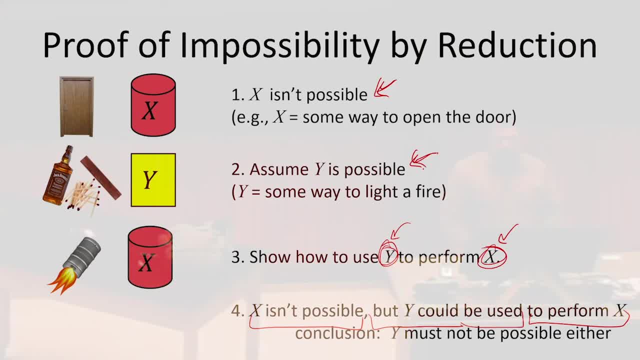 then if we had assumed that it was possible for him to light a fire, since he could have used that fire to open the door, our conclusion is: the fire wasn't possible. Basically, the reason that it becomes a proof by contradiction is because of step two. 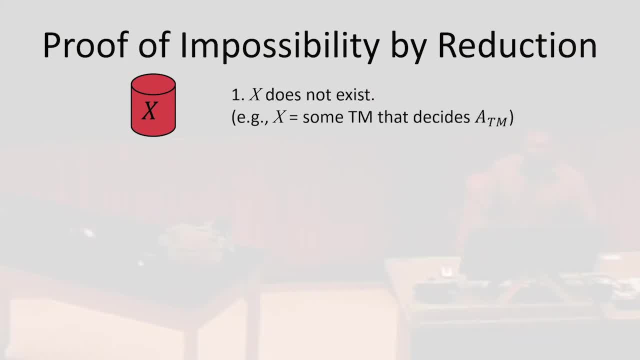 We assumed something that was, that was false. So what we're going to do is I'm going to show you how we can use this idea. We're going to show how we can, how we can show in a different way that the halting function is not computable. 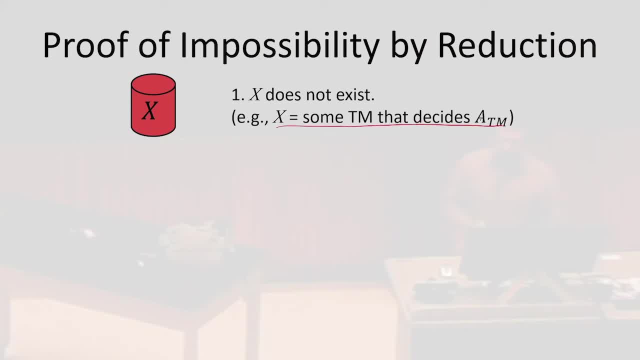 Walking in the door we knew that there was not a Turing machine to decide the acceptance function for us. So ATM was that acceptance language. So there is not a Turing machine that could do that acceptance problem for us, that could solve the acceptance problem for us. 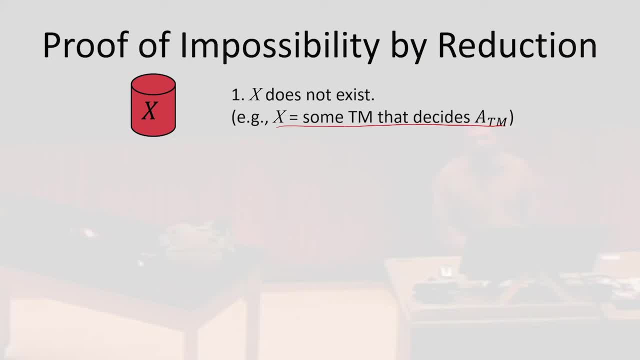 So we know that already. We have proven that independently of anything else. We just know that to be a fact. So let's assume, towards reaching a contradiction, that is, that I have some Turing machine that's going to decide the problem B. 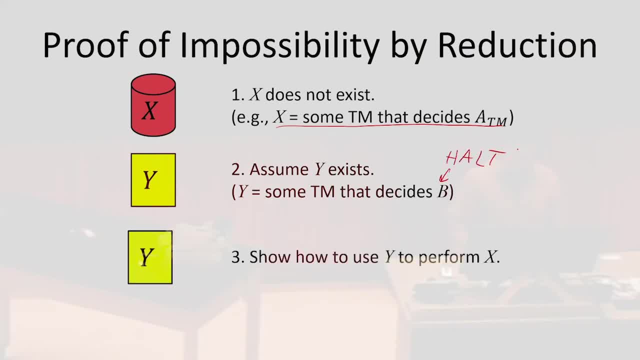 which I'm going to say is the halting problem. So let's say that problem B is the halting problem and I have some Turing machine that's going to decide it. What I'm going to do is I'm going to show how I could use this solution to halt. 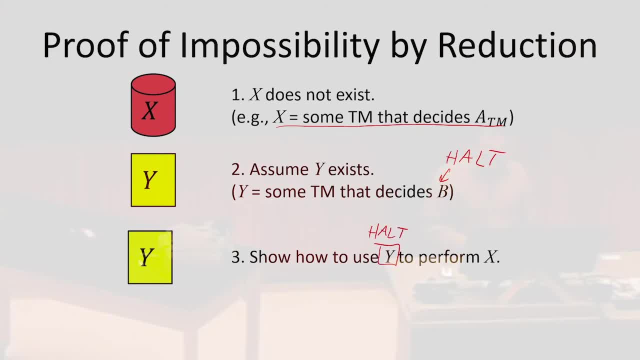 In order to make a solution for the acceptance problem. I'm just going to describe some method where if, hypothetically, I had a function or I had a Python program or a Turing machine that could compute halt for me, I could use that to compute the acceptance problem for me. 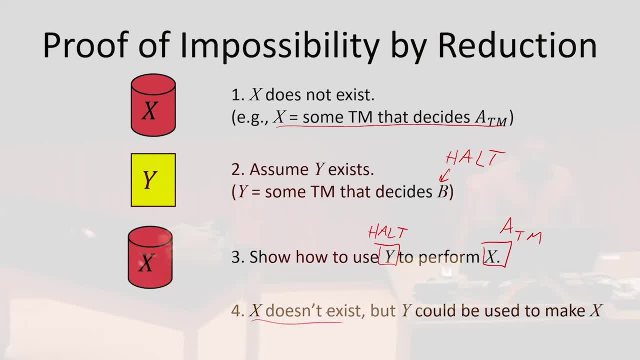 Whatever method that looks like, since we knew X didn't exist, there wasn't anything that could decide ATM, that acceptance problem for us. But we could use this solution to the halting problem to make a solution to the acceptance problem. Our conclusion must be that we couldn't have actually built. 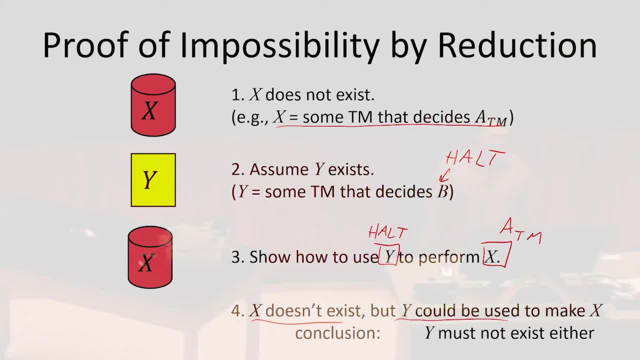 that solution to the halting problem. So we're going to use our knowledge that ATM was impossible to solve in order to demonstrate that halt was impossible to solve. So we've already shown that halt was impossible to solve. We're just going to prove it. 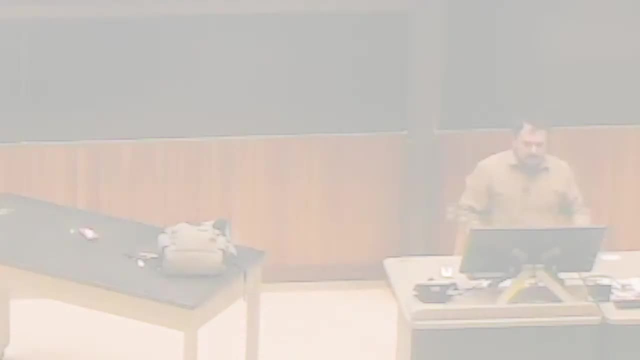 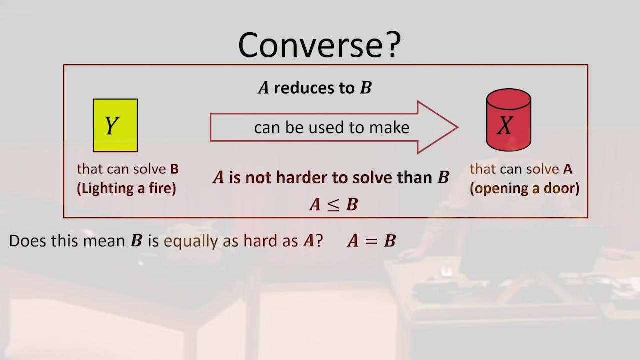 in a different way. now, Before we carry on, let's consider the opposite. So let's explore this technique, the powers and limitations of this reduction technique, a little bit. So what we did is we showed that a solution to this problem of lighting a fire. 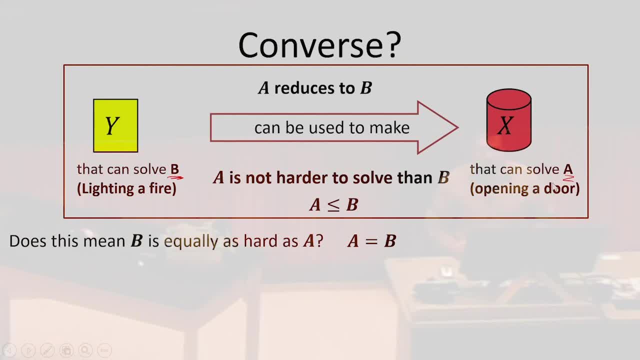 could be used to make a solution to this other problem: opening a door. Does this mean that they're equally as difficult? So the question is: what about the opposite? Does this mean that if I have a problem, if I could open a door? so we showed? 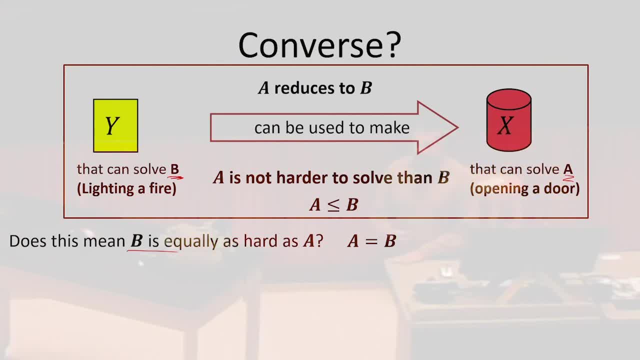 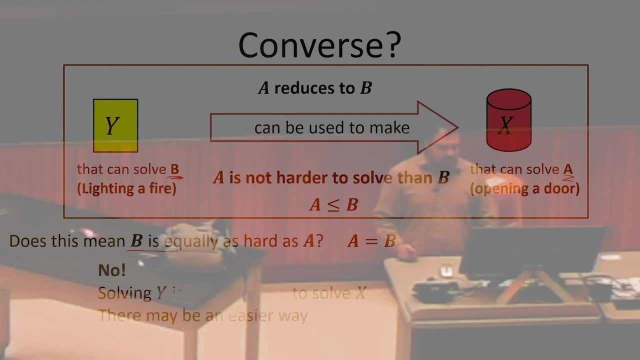 that if I can light a fire I can open a door. does this mean if I could open a door, then I could light a fire? Yeah, so the answer is no. I'm seeing lots of this because there's lots of ways to open doors. 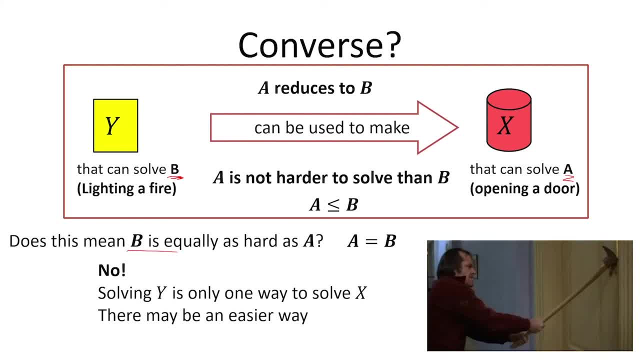 For instance, I could use an axe. If there was an axe in the room then I didn't need MacGyver to light a fire in order to be able to open that door. So there might be other ways besides solving problem B. 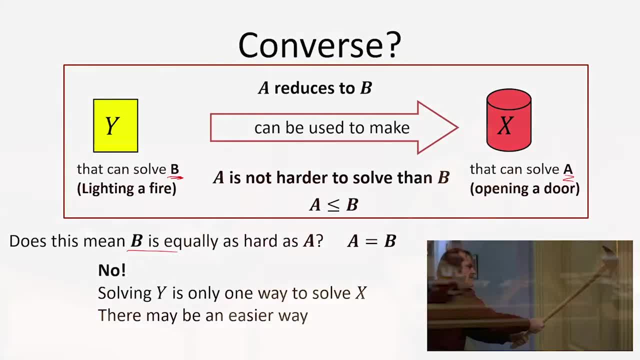 in order to solve A. So this does not mean that MacGyver would be able to open a door. So this does not mean that MacGyver would be able to open a door does not mean that they're equally difficult. 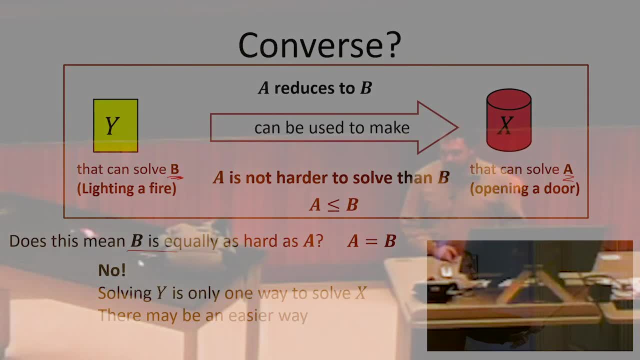 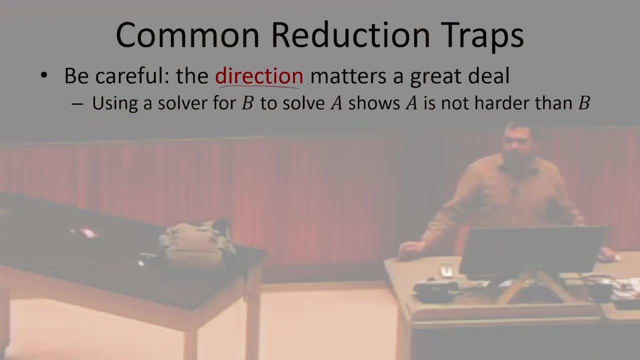 This does not mean that the opposite is going to be true as well. This only works in one direction. is the important thing here? Also, be careful about the direction. A lot of what you're gonna see, a lot of the notation seems to be counterintuitive. 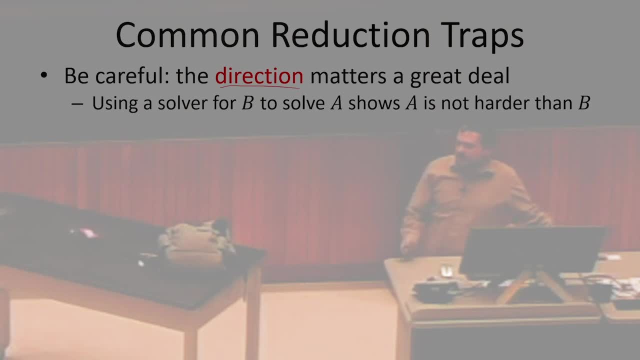 Something to keep in mind is that when you see less than or equal to, you're comparing the hardness of two different problems. So let's say that I'm using a solver for problem B in order to solve problem A, showing that A is not harder than B. 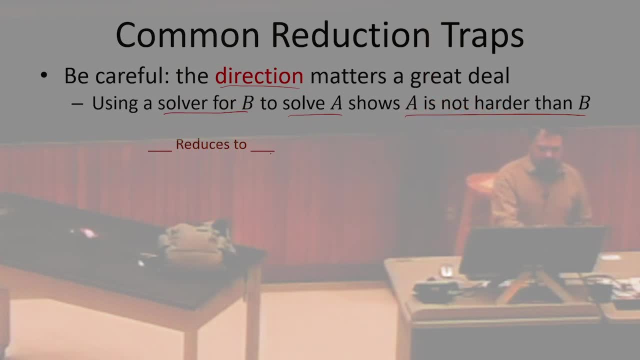 What reduces to what? Fill in the blank with A and B. in these two blanks, Which one is which? So, in this case, we're using a method for solving B in order to produce a method for solving A. Which one's the door, which one's the fire? 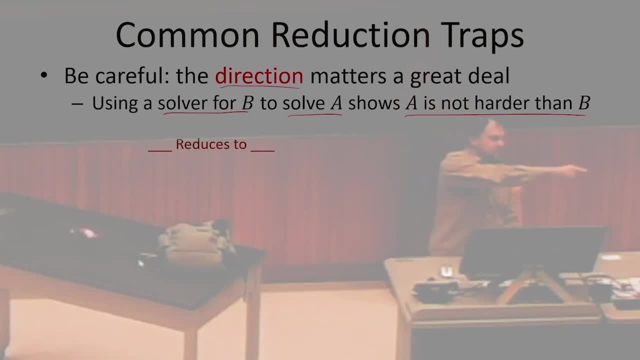 So which one's the door? Yeah, which one's the door? We're using a solver for B to solve A. So the end problem we're trying to solve is A. So that's the door And B is going to be the fire. 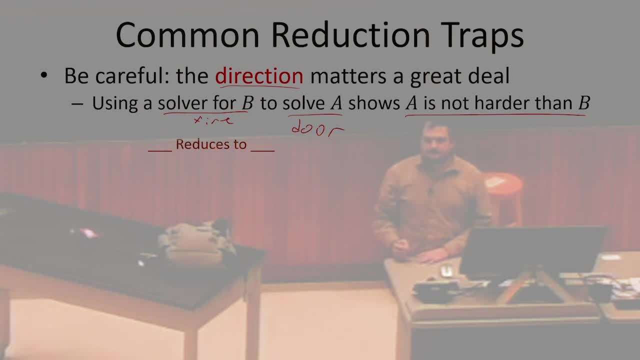 So what reduces to what? Yes, So we're gonna say: A reduces to B, The problem of opening a door reduces to the problem of lighting a fire. Something else to keep in mind is that your transformation must only be things that you can do. 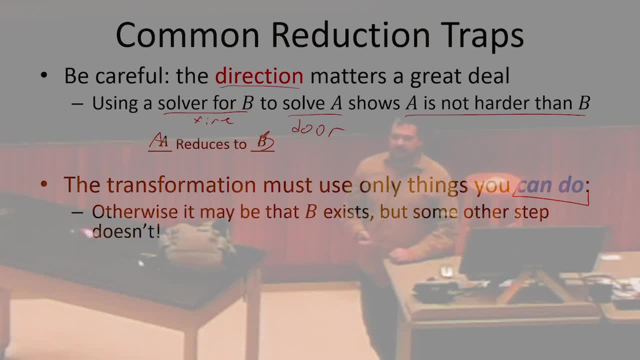 Your transformation must only be things that you can do. Your transformation must only be things that you can do, That are permitted for you to do. Basically, in this case, what can do means is anything that you can do with a Turing machine that always holds. 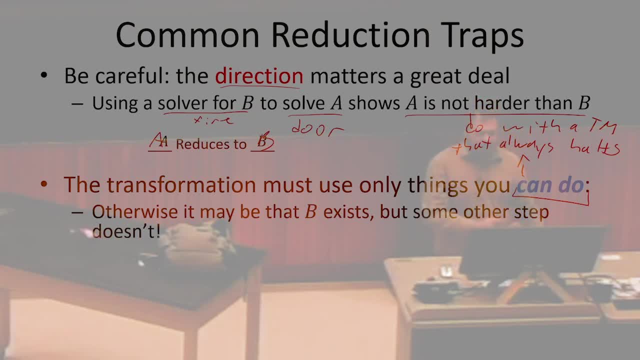 Reductions can be used for lots and lots and lots of different things. If you haven't already, you will see also reductions in your algorithms class. We're gonna be using them again for another topic later this semester as well. The thing that you can do changes on your application. 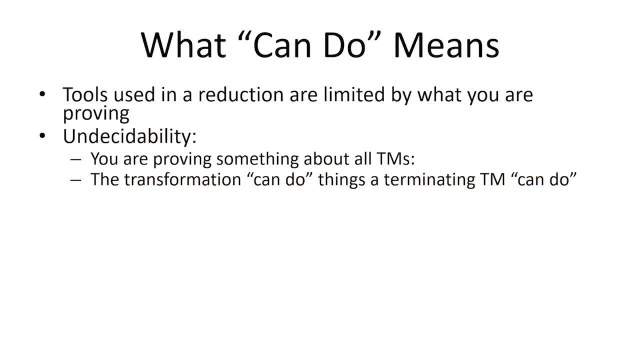 for this application. you're allowed to do anything that a Turing machine can do and hold.